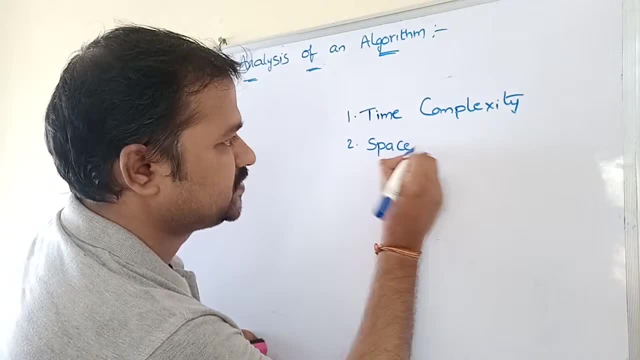 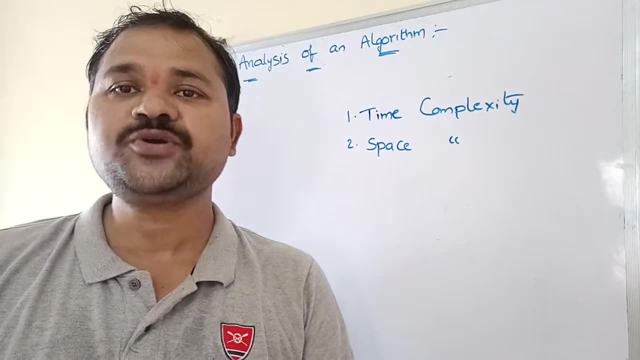 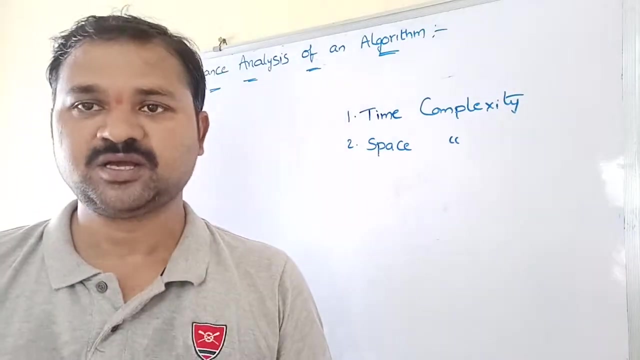 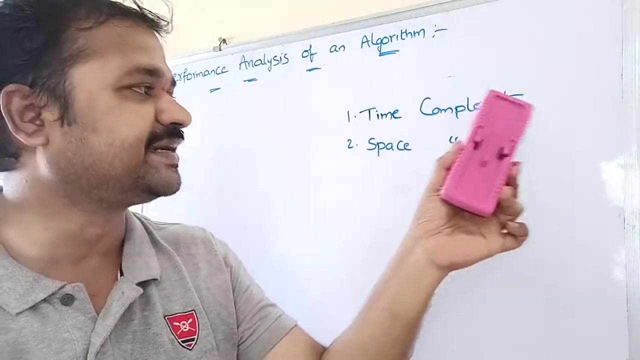 Space complexity. So first let's see about time complexity. First let's see the definition of time complexity. The amount of time that an algorithm requires for its execution is known as time complexity. So how much time that an algorithm requires for its execution is nothing but time complexity. 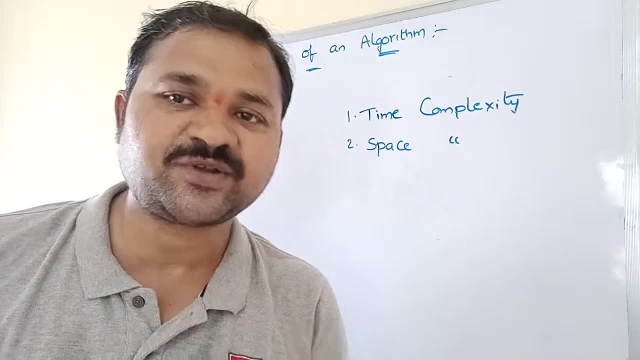 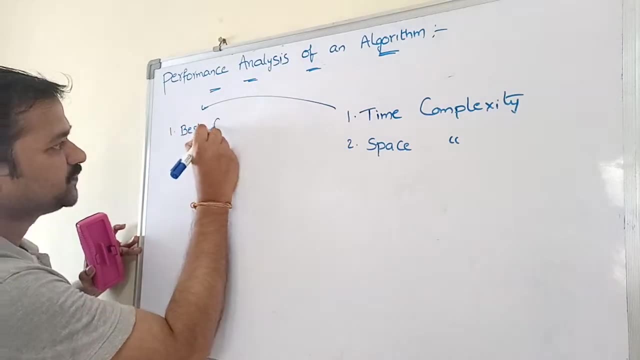 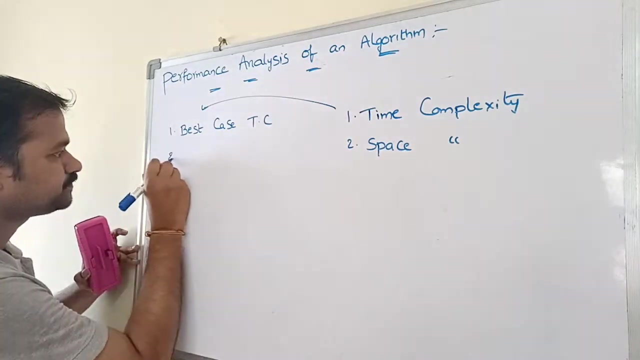 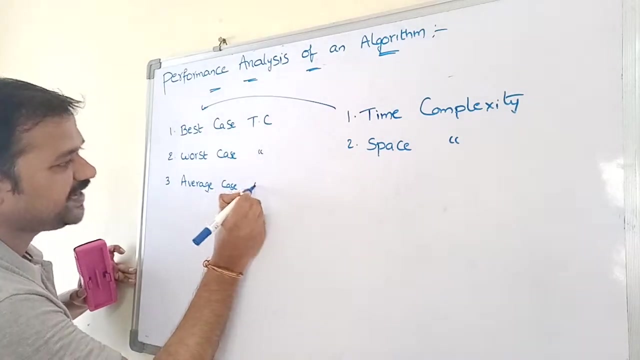 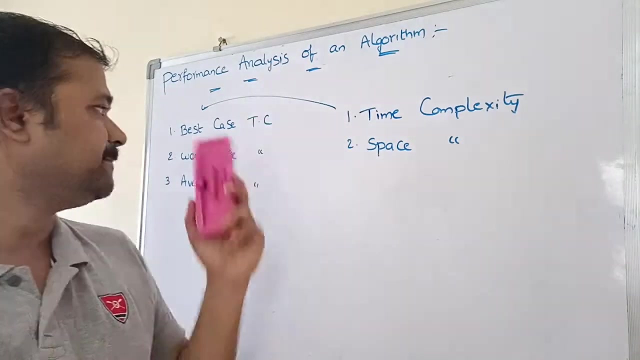 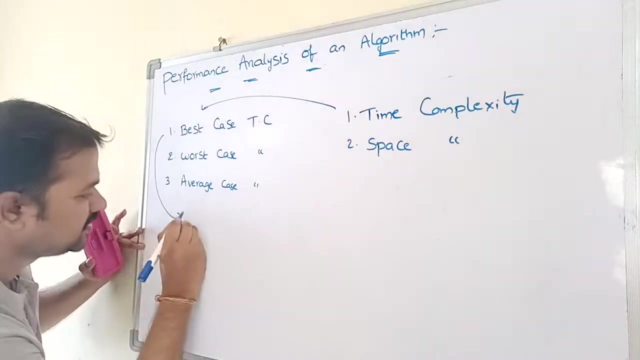 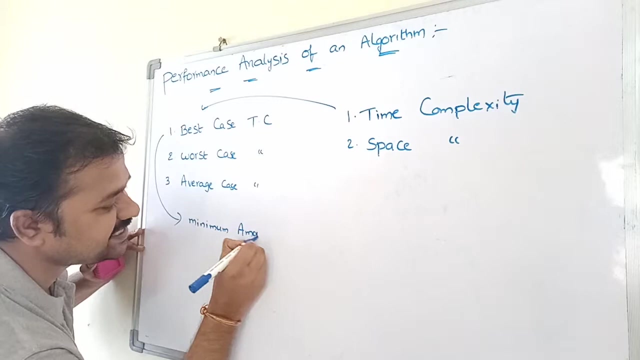 There are mainly three types of time complexities are available. The first one is best case time complexity. Second one is worst case time complexity. Third one is average case time complexity. So we have three types of time complexities: Best case, worst case, average case. Now let's see about best case time complexity If an algorithm requires minimum amount of time. if an algorithm requires minimum amount of time for its execution, then it is known as best case time complexity. 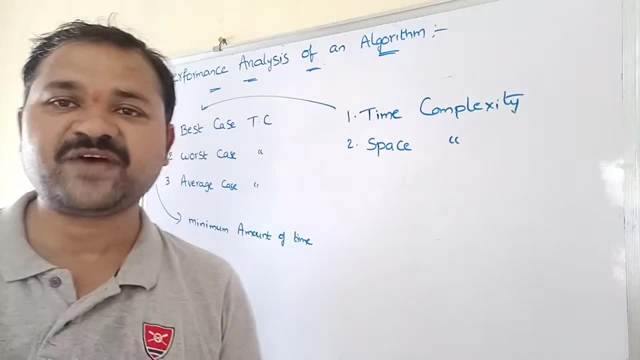 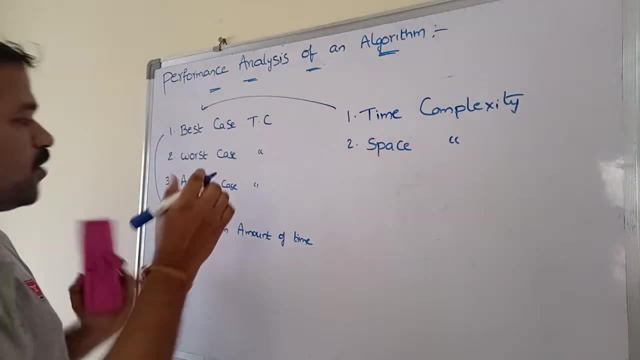 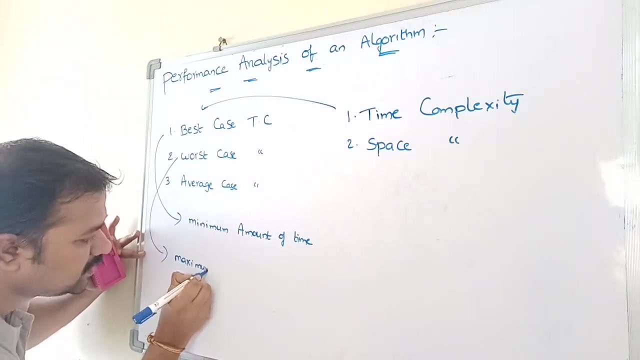 So best case means algorithm requires minimum amount of time for its execution. Now let's see what is worst case time complexity If an algorithm requires maximum amount of time. if an algorithm requires maximum amount of time for its execution, then it is known as worst case time complexity. 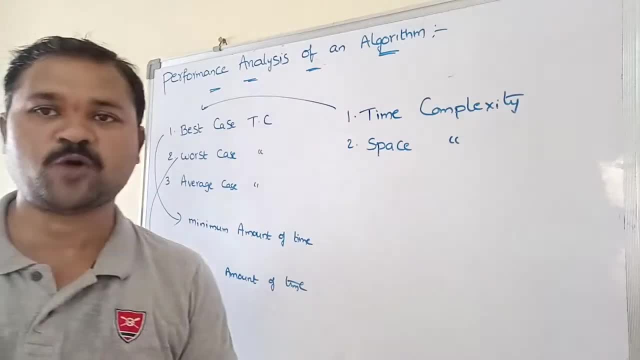 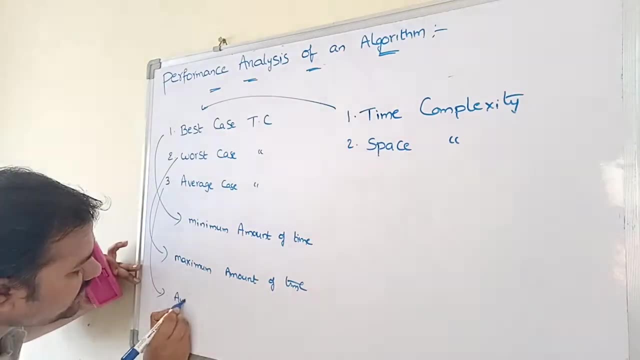 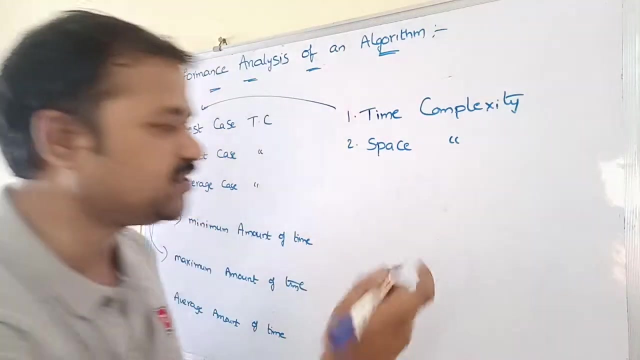 Now let's see what is average case time complexity. If an algorithm requires average amount of time for its execution, then it is known as worst case time complexity. Now let's see an example for best case, worst case and average case. Before that, let's see what is linear search. 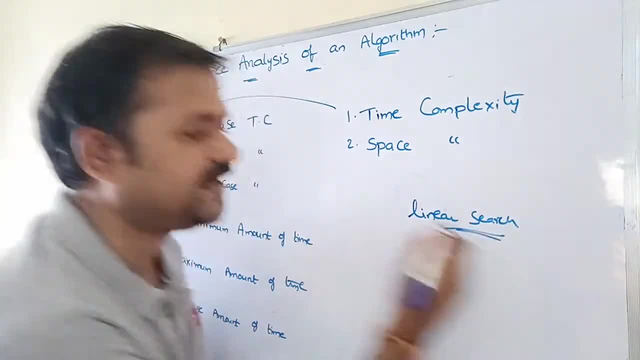 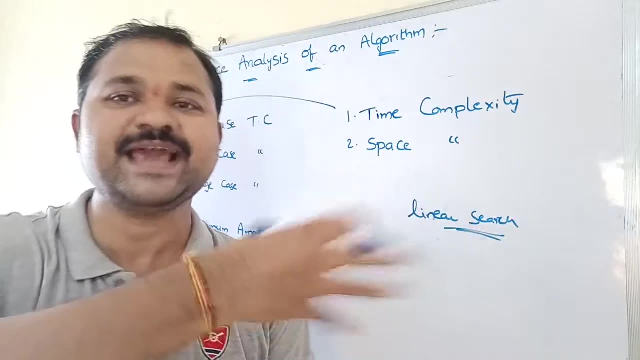 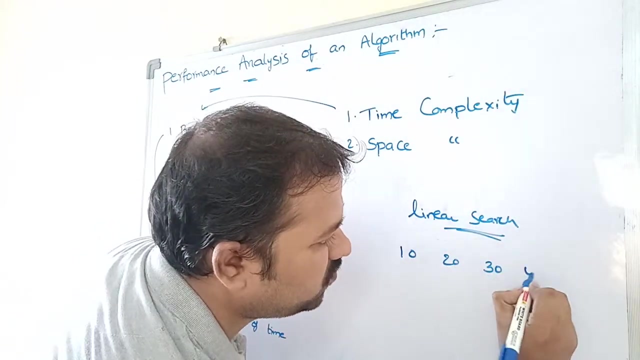 So linear search means searching the elements of the list one by one until the key element is found or the array is completely exhausted. The array is completed. Elements of the list are some 10,, 20,, 30,, 40,, 50, various. the key element is 40.. 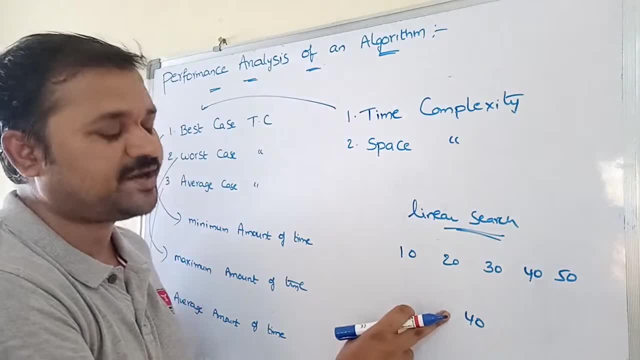 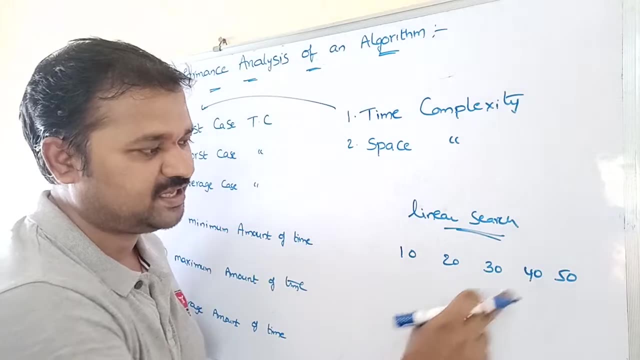 So first we have to compare 10 with 40. So not equal. So compare 20 with 40, not equal. So compare 30 with 40, not equal. Next, to compare 40 with 40, equal. 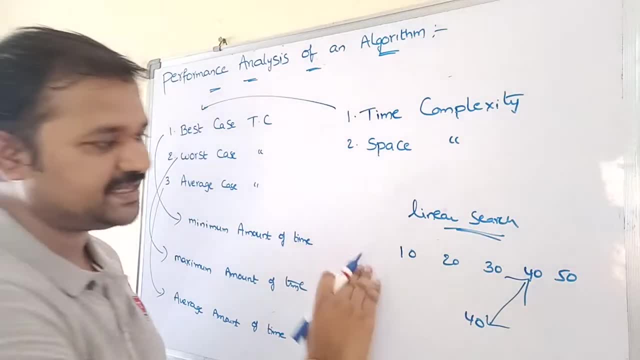 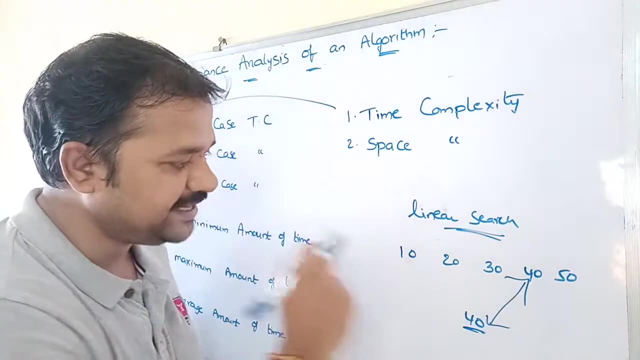 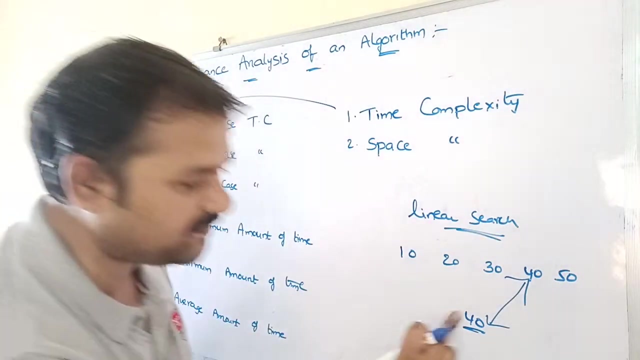 So we can say that the key element is found. So these are nothing but elements of the array or elements of the list. So this is nothing but key element. So compare key element with elements of the array one by one. until the key element is found or the array is exhausted, the array is completed. 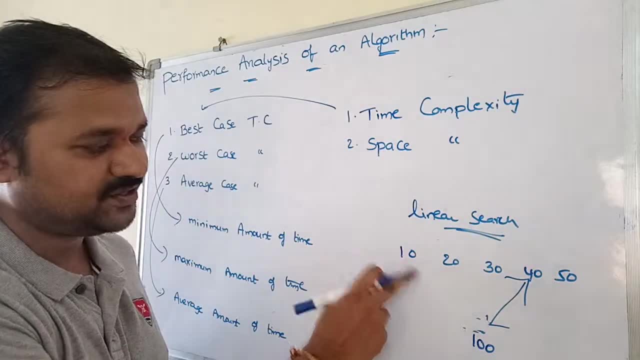 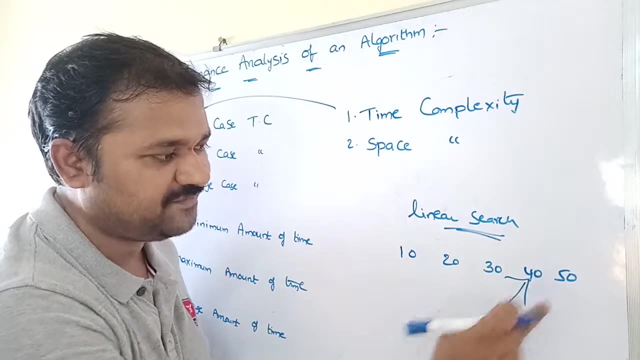 So let the key element here is 100.. So 10, 100, not equal 20, 100, not equal 30, 100, not equal 40, 100, not equal 50, 100, not equal. 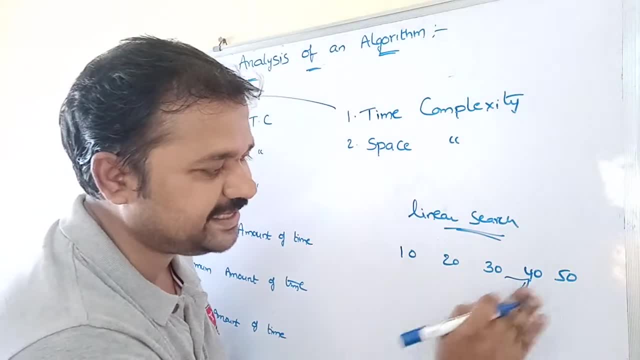 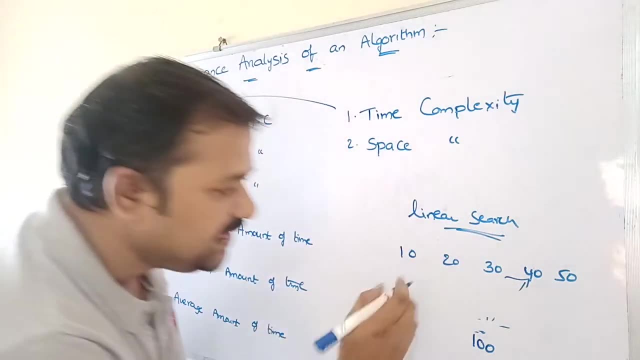 Array is exhausted. Array is completed. So we can say that here the key element is not found. So while searching an element Using linear set, If the key element found at first position, Let, the key element is 10.. So compare 10 with 10.. 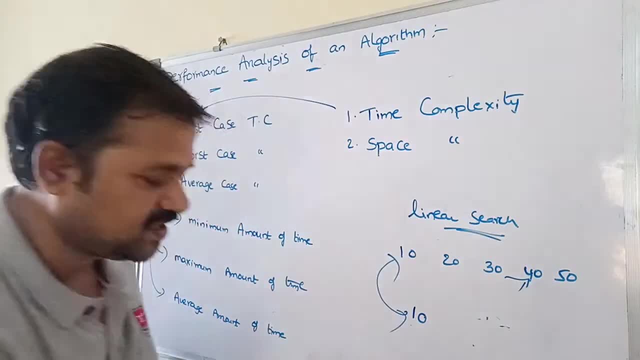 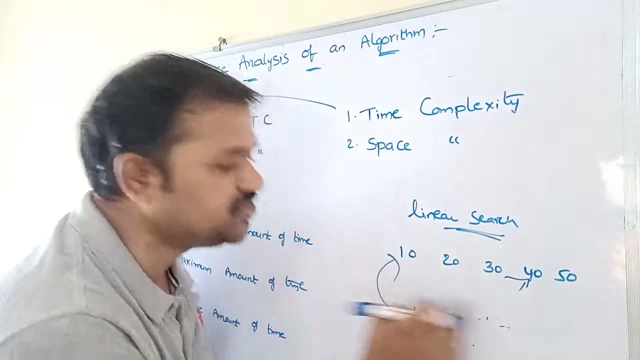 Both are equal, So this is nothing but best case. So, while searching an element Using linear set, If the key element found at first position, Then it is called as best case 10 complexity. Why? Because what is best case? 10 complexity. 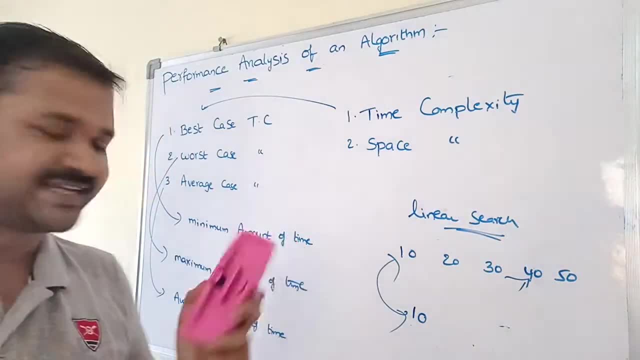 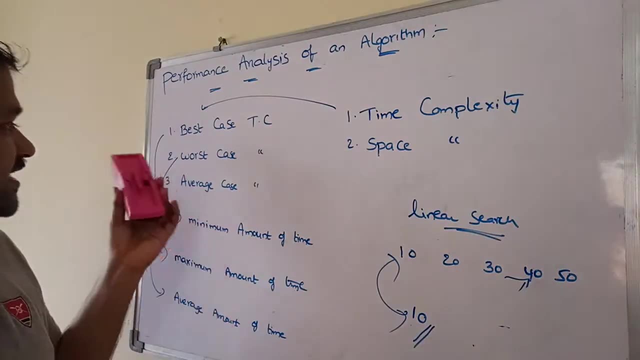 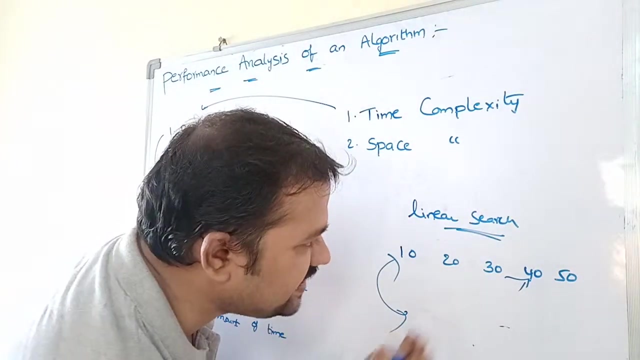 Algorithm requires minimum amount of time For its execution, So here we need only one unit of time For comparing the element. Now let us see an example for worst case 10 complexity While searching an element using linear set, If the key element requires maximum amount of time. 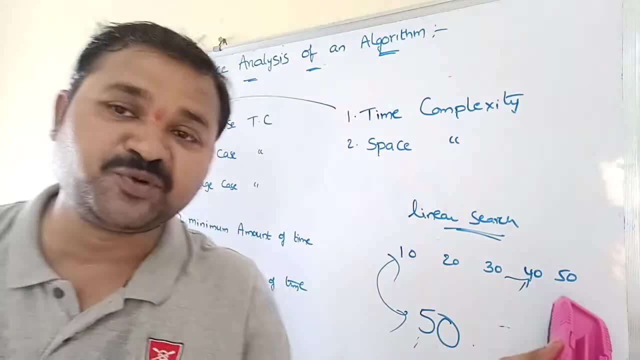 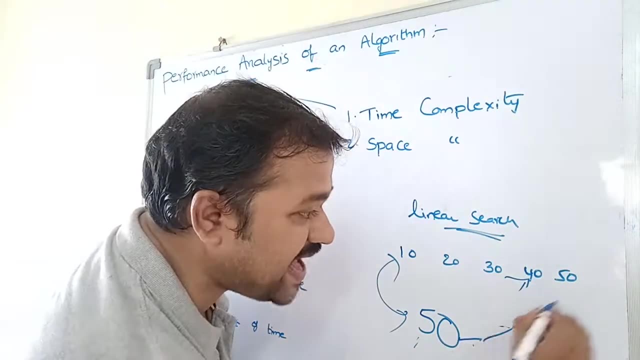 That means if the key element found at last position While searching an element using linear set. If the key element found at last position, Then it is called as best case- 10 complexity. Then it is called as worst case- 10 complexity. 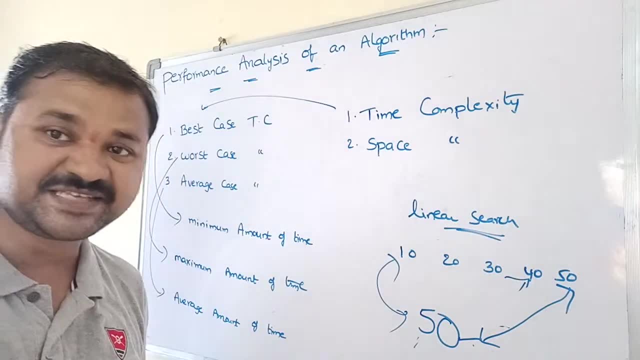 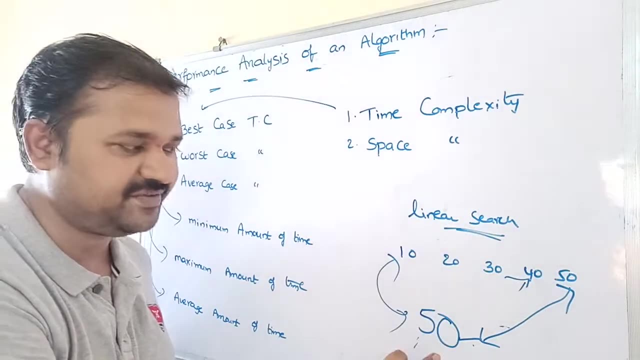 Why? Because worst case means algorithm requires maximum amount of time for its execution. So here, what is the maximum amount of time? 5 units of time. So 1050 not equal. 2050 not equal, 3050 not equal. 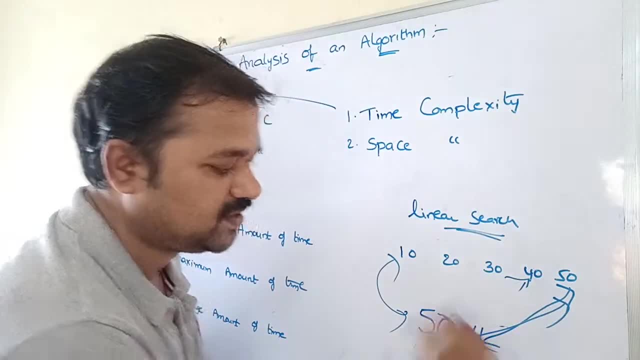 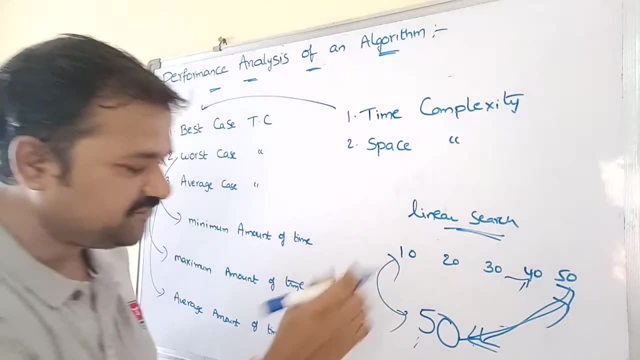 4050, not equal 5050.. So they are equal. So we can say that this is the best example for worst case. So what is the best example for best case If the key element found at first position? 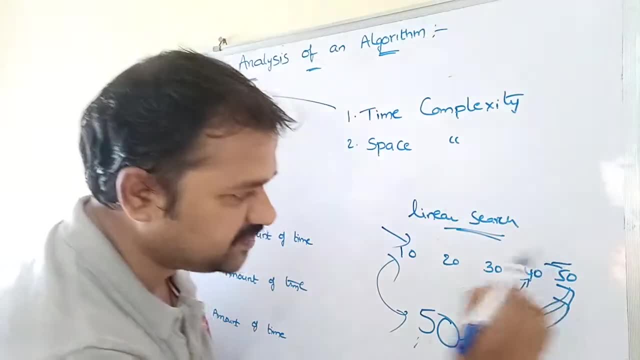 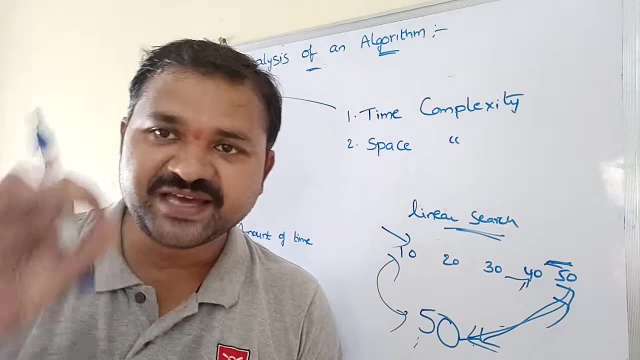 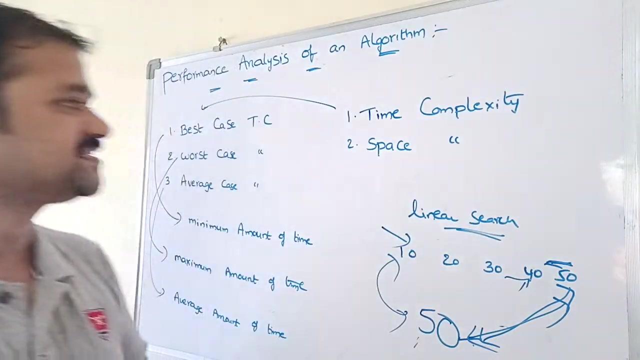 Then it is best case. What is worst case? If the key element found at last position, Then it is worst case. Next, the average case means If the key element found at some second place or third place or fourth place, Then we can say that it is some average case. 10 complexity. 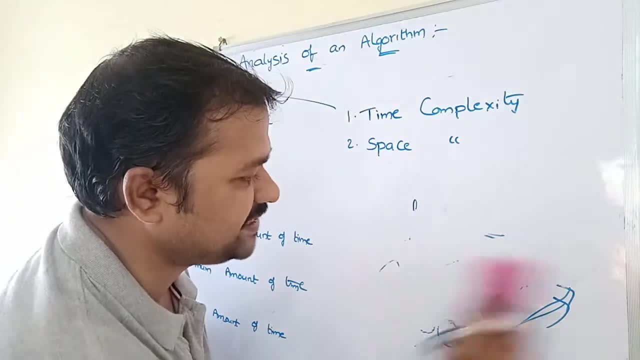 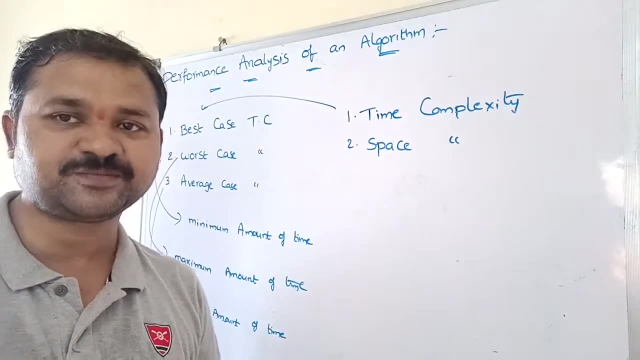 So this is about different types of 10 complexities. So best case, What is best case? 10 complexity While searching an element using linear set. If the key element found at first position, then it is best case if the key element 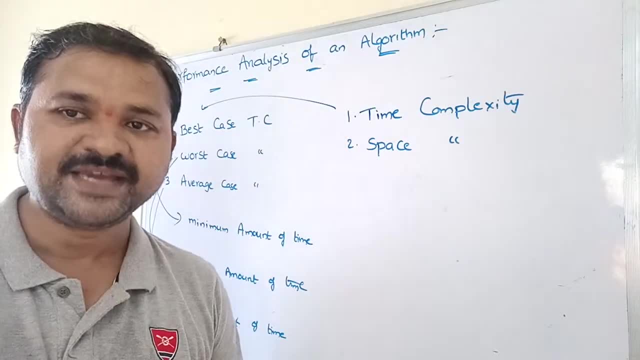 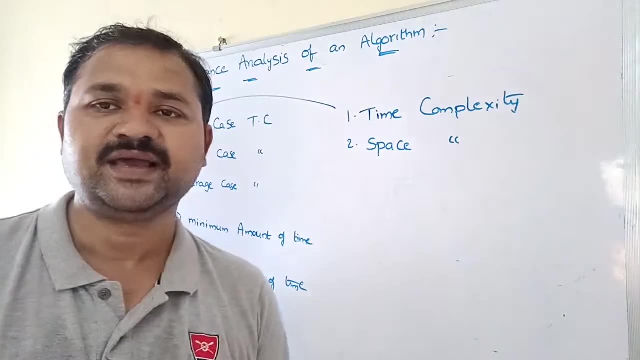 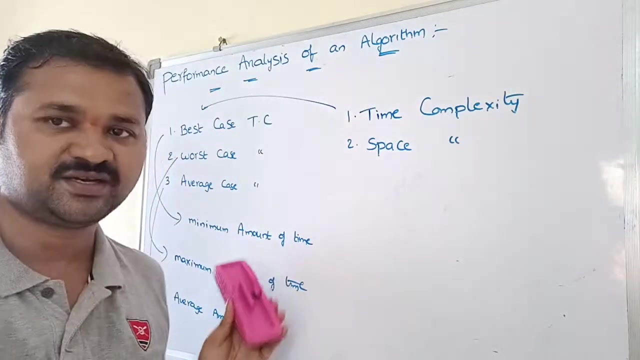 found at last position, then it is worst case. if the key element found at some middle position- it may be some second position or third position or fourth position- then it is nothing but average case. 10 complexity, So best case means algorithm requires minimum time for its execution. 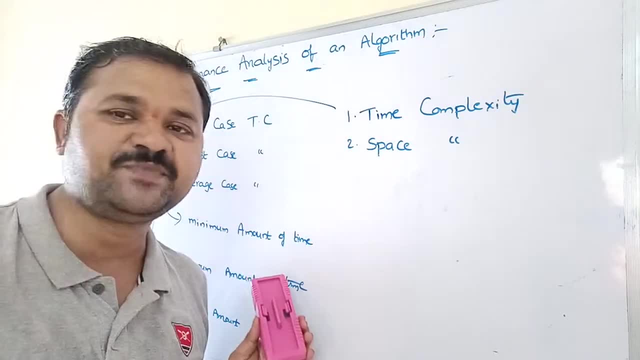 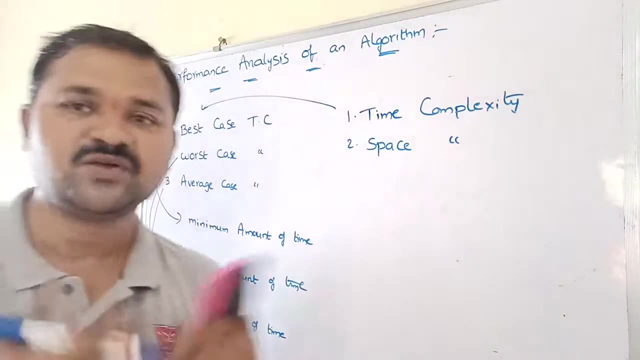 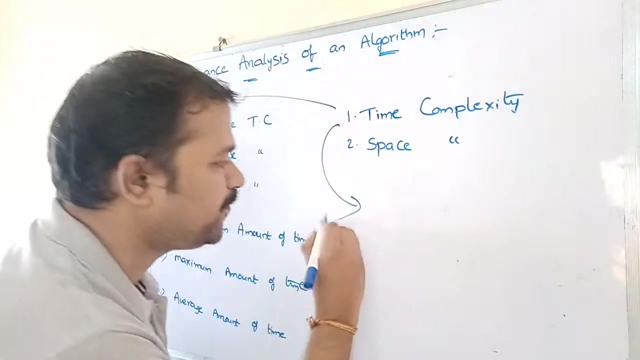 Worst case means algorithm requires maximum time for its execution. Average case 10: complexity. Worst case means algorithm requires max average amount of time for its execution. In order to calculate time complexity, we have two approaches. The first approach is frequency count or step count. 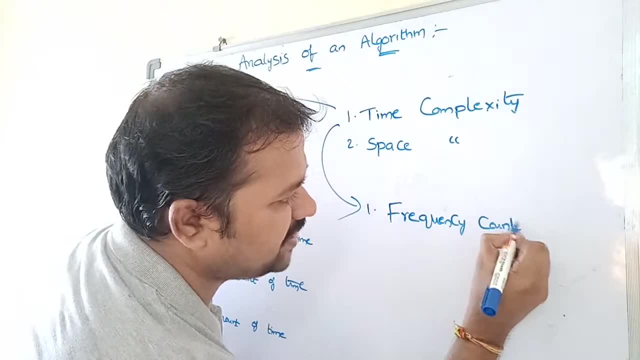 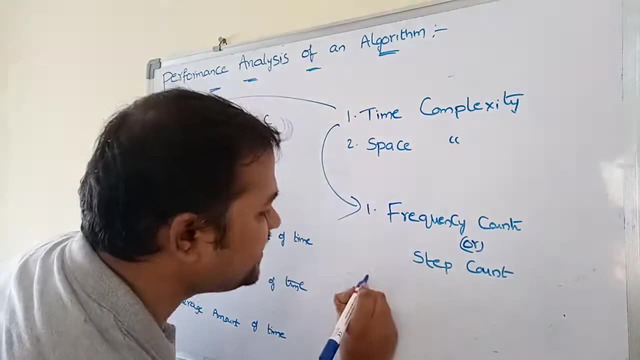 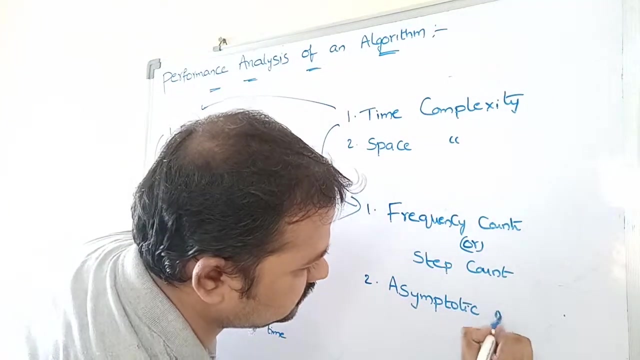 So there are two approaches in order to calculate time complexity. The first one is frequency count or step count, Whereas the second approach is asymptotic notations. The second approach is asymptotic notations, So we can calculate time complexity using two approaches. 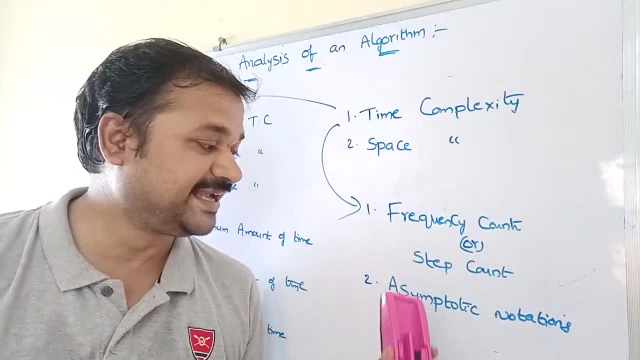 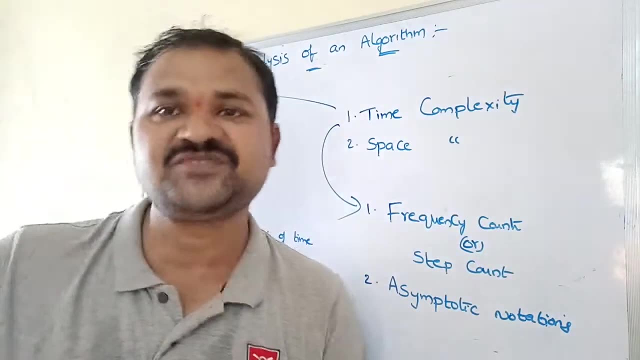 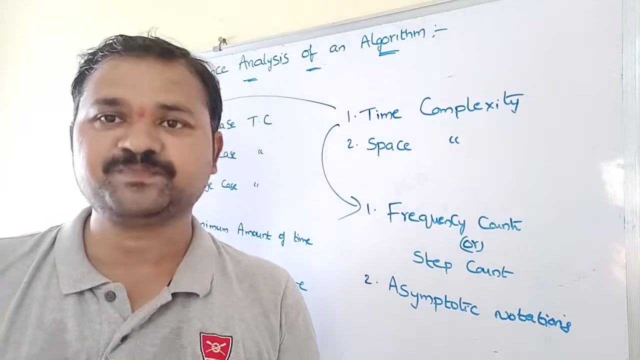 First one: frequency count or step count. Second one: asymptotic notations. We will discuss about frequency count and asymptotic notations in the next videos. Now let us see what is space complexity. What is time complexity? The amount of time that an algorithm requires for its execution. 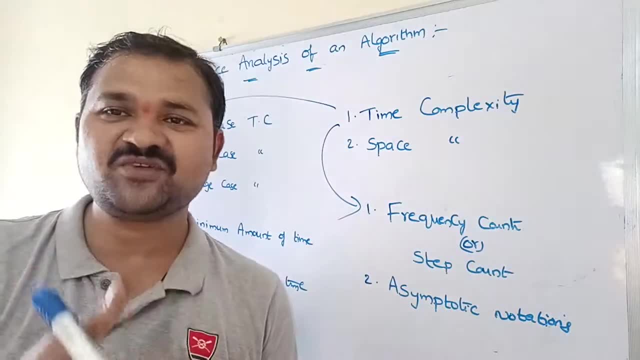 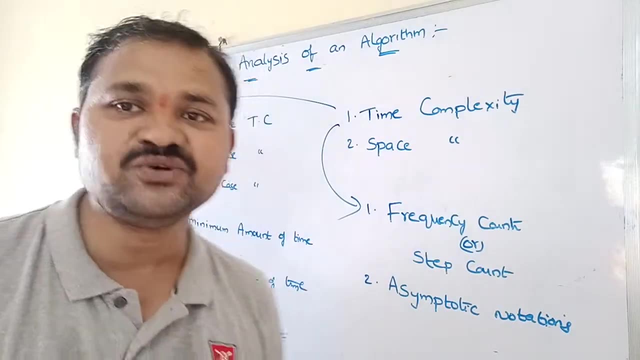 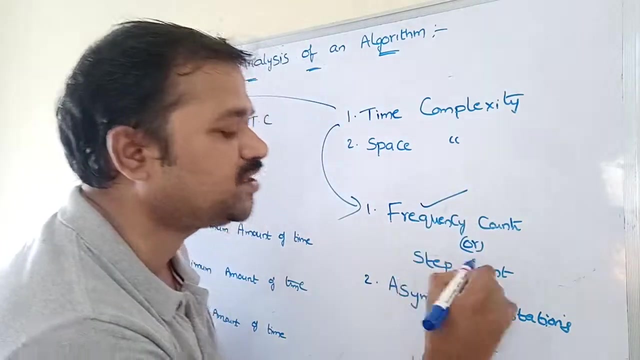 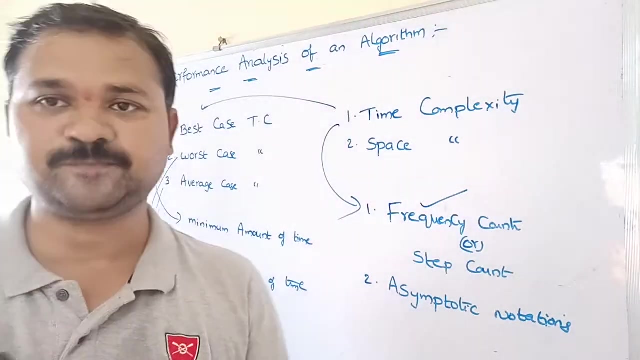 So various space complexity means: in place of time, we need to write space. So the amount of space that an algorithm requires for its execution is known as space complexity. We will discuss how to calculate space complexity in frequency count or step count approaches. So this is about performance of performance analysis of an algorithm. 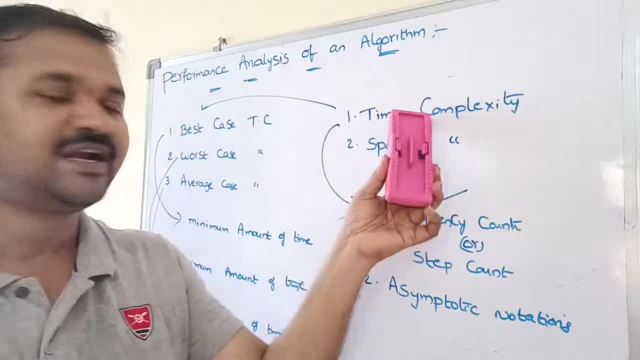 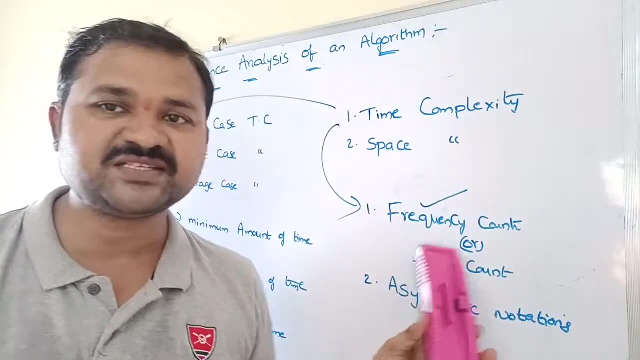 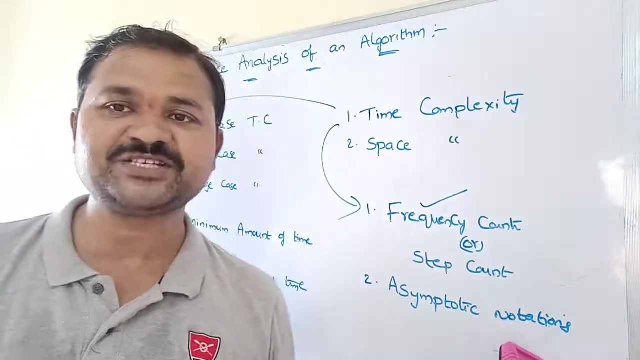 So we can analyze performance of an algorithm using time complexity as well as space complexity. Again, we can calculate time complexity using two approaches: frequency count or step count and asymptotic notations. So we will discuss about frequency count and asymptotic notations in the next videos. 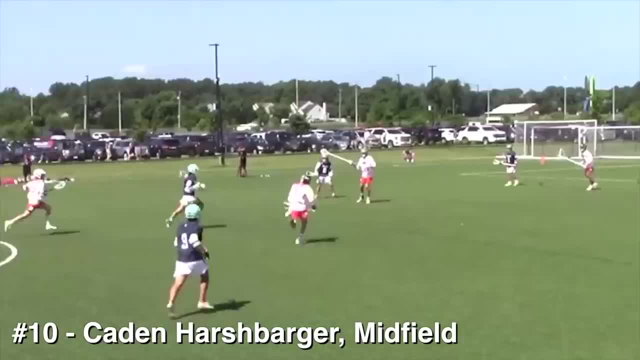 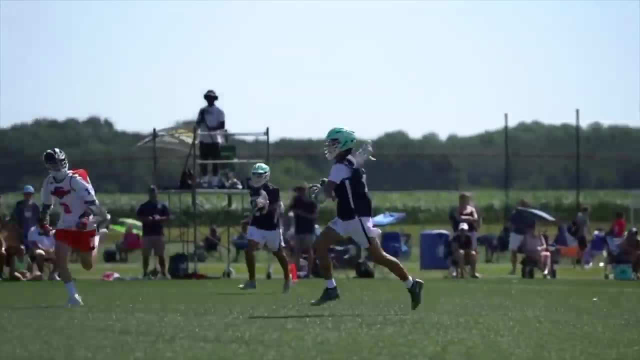 So the top 10 lacrosse recruits in the class of 2024, starting with number 10, Caden Harshbarger, a midfielder from Lake Mary Florida Athletic, is the first word that comes to mind when you watch this guy play, Whether it's a shot down the alley or a defensive stand. 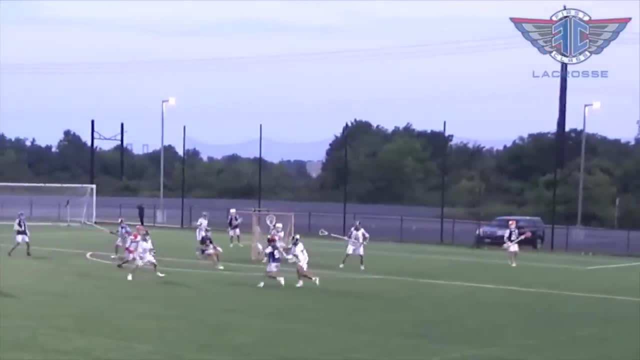 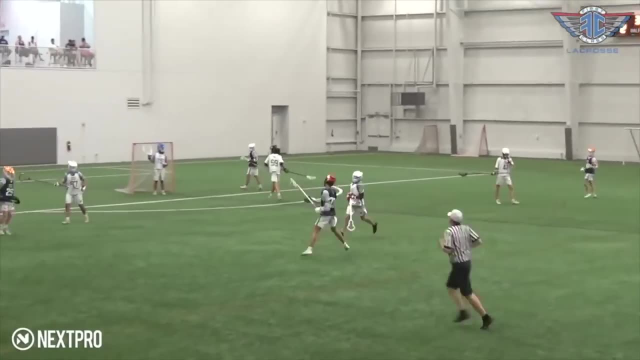 at the end of the game. he can make plays all over the field. At 6 feet tall and 175 pounds, Harshbarger has all the physical capabilities that D1 lacrosse coaches rave about. His ability to shoot the ball from the outside but also use his quickness on the inside makes him a special. 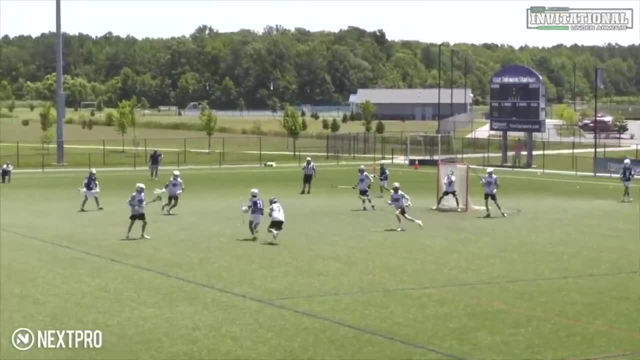 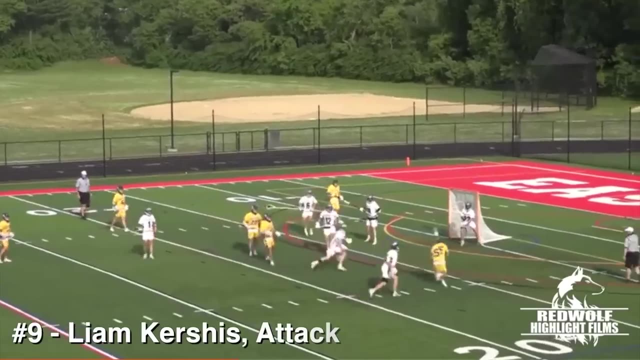 player, And his phone will be ringing off the hook in September. I'm excited to see where Harshbarger plays college lacrosse and I just know that we'll be seeing him on ESPNU soon. And next up, at number 9, we have Liam Kershis, an attackman from Shoreham Waiting River in Long Island. This guy 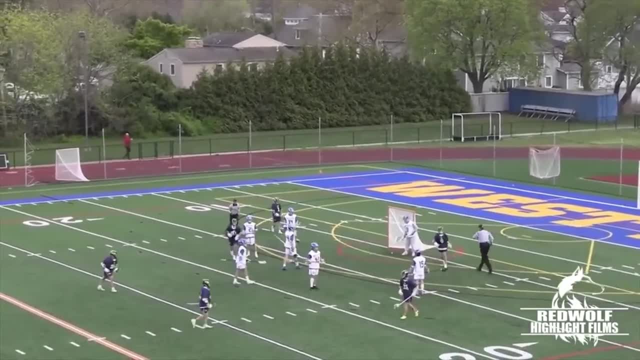 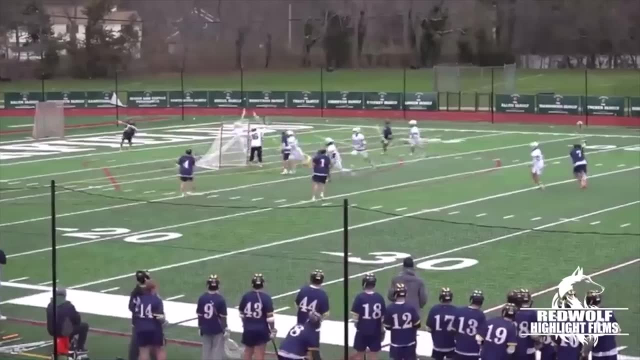 makes a living at X picking apart defenses and getting to the cage if he needs to. He always has his head up, which makes it so tough for defenders to know if he's about to pass or shoot. But calling Liam just an ex-attackman would be doing his game a disservice. You can see this. 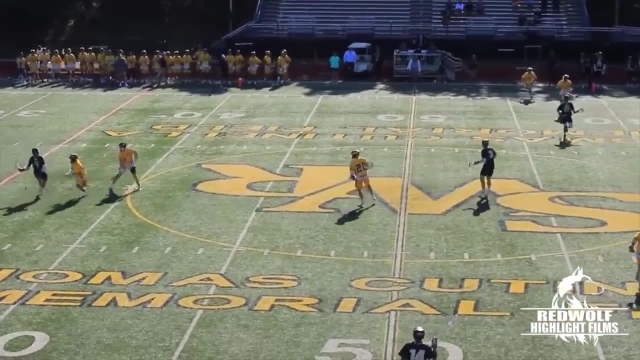 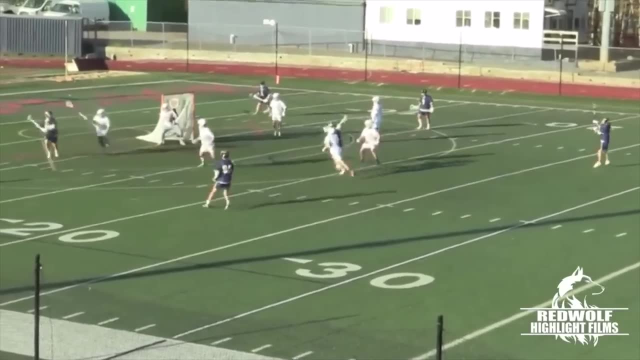 man make plays all over the field. In his highlights you can see him multiple times getting the ball back on the ride, and he's also deadly from the wing, so you can't just play him in one place. I think he's a lefty, but he also scores at will with his right hand, which makes 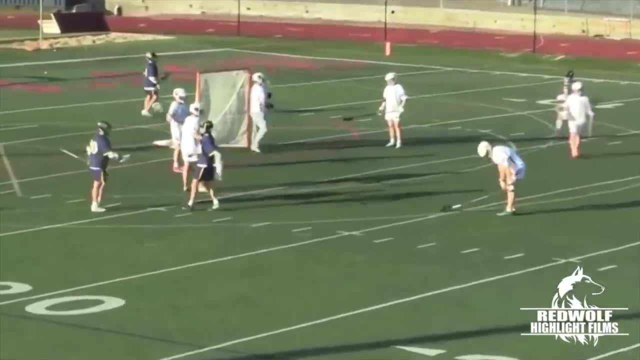 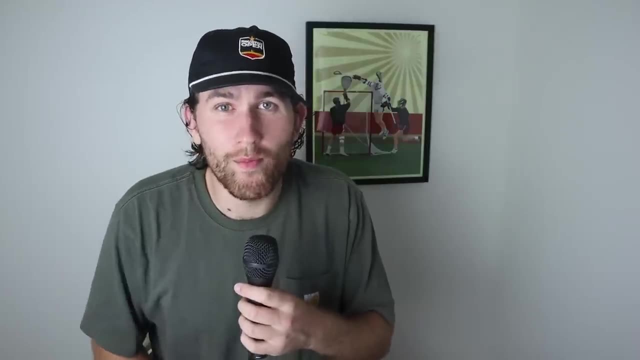 him a matchup nightmare, however you try to play him. His coach says he's one of the most cerebral attackmen he's ever coached and you can clearly see why in his highlights He reminds me a lot of another Shoreham Waiting River alum, Chris Graham. 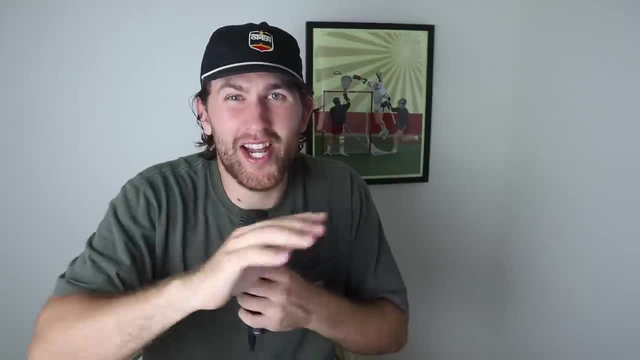 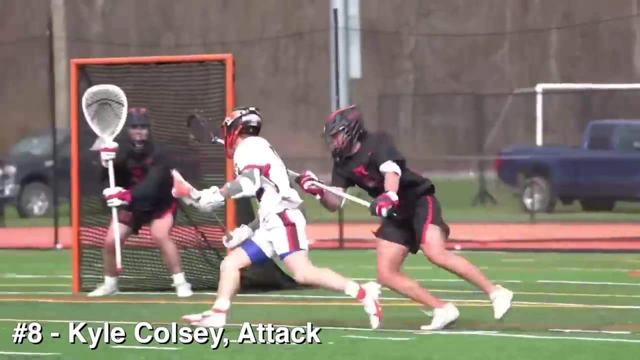 He was absolutely tearing it up in the PLL. I think Liam projects extremely well at the next level And at number 8, we have Kyle Colesie, an attackman out of Richfield, Connecticut. The first thing you notice about Kyle is that he plays a million miles an hour. He has one speed and it's.